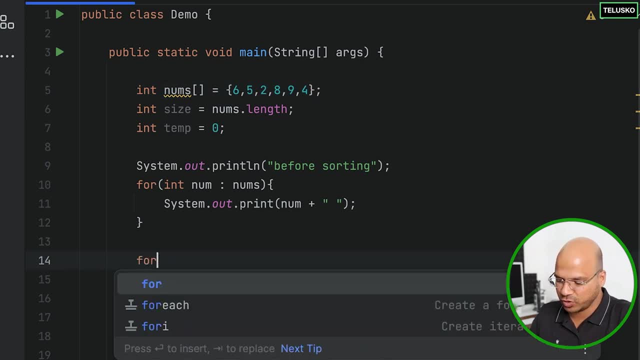 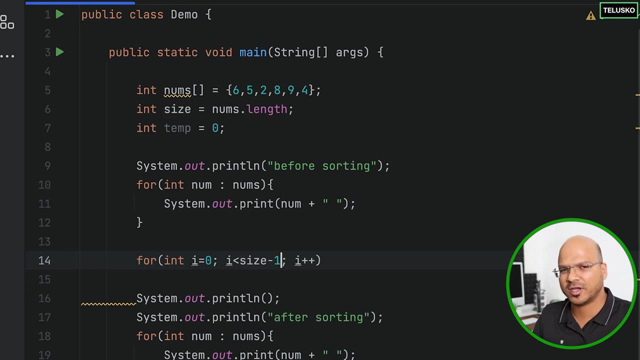 first value and that's how we can start. And for doing that we have to use two loops: the outer loop and inner loop. We'll start outer loop with zero and then we'll say i less than size, right, Okay? so we'll say i plus plus. but also we can make it more efficient by saying that size minus one is because if you remember when we were doing the sorting, and once you got all the values sorted except the first value or the last value, you don't basically sort the one value, right, So you can reduce the number of iterations. 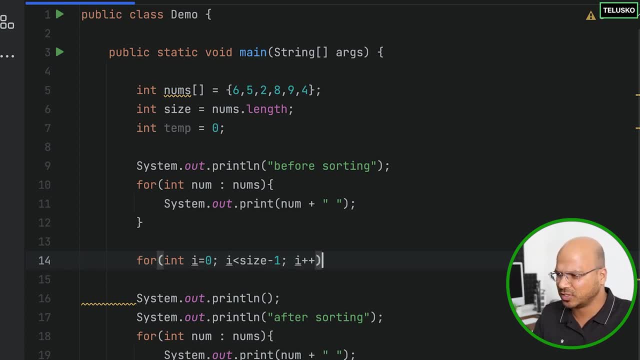 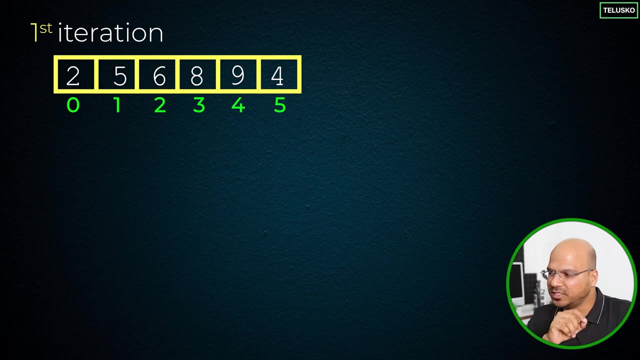 you go for. So we can say size minus one and we'll see if that works or not. and if it works, then we are happy. We'll also go for the inner loop. Now for the inner loop, we'll go for j equal to Now. where do we are going to start j? So basically, if you're putting the starting, the biggest value or the smallest value at the start, what it means is, after for every iteration, the inner loop, we can skip the first value, right. So for the second iteration we can skip the first value. For the third iteration, we can skip the first two values because they are sorted. 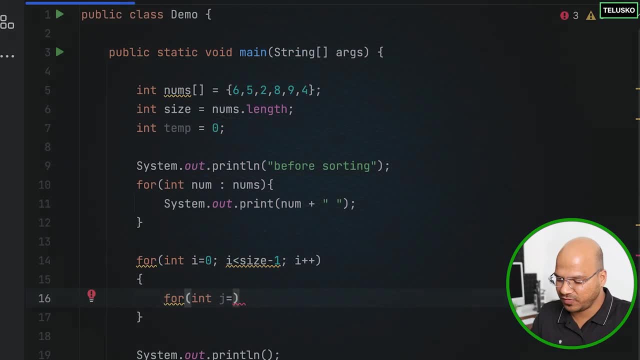 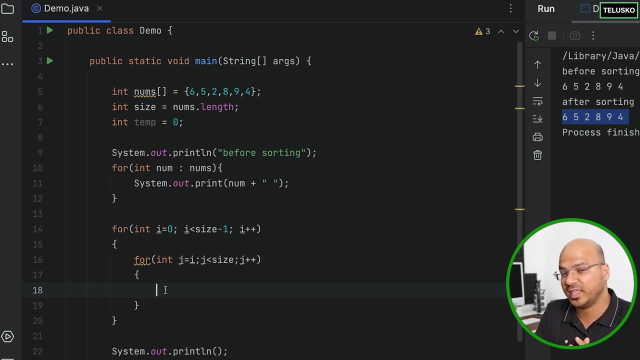 Right, so we have two sections right: sorted array and unsorted array. So here we can start with j equal to i. Yeah, in fact, when your i value is zero, j should start from zero. So we can say j equal to i and j less than size and j plus plus. So basically we have to, we have to go to the end, Okay, so that's the for loop. we have Now what you do inside this. So we have to find the minimum value To start with. we can take min value variable here, So I can say int. 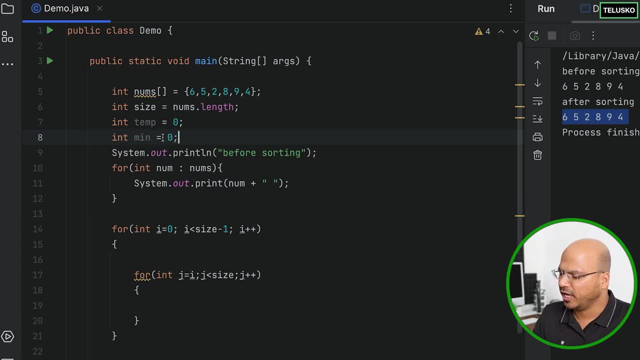 min is equal to zero. In fact, we want the min index, not the min value, because we have to work with the index, right? And we'll say the index is by default minus one. And here, to start with, we'll start with min index equal to i. And then what you do? you basically check if the array which is nums of min index. Now we want this to be smallest value, right? So I assume that this is the smallest. but what if this is not the smallest compared to the 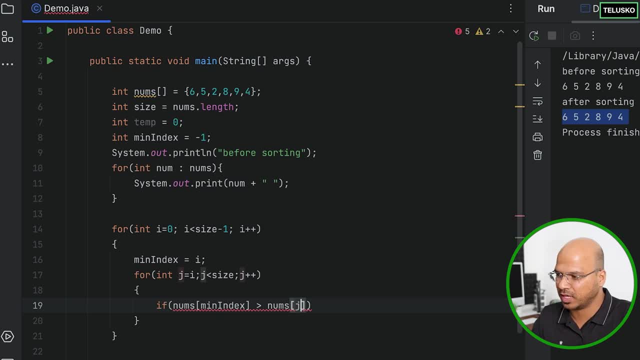 value which we are considering. The value which is considering here is nums of j. So, example: if this six is the smallest, which we are thinking, In fact you know, we should be saying i plus one, The reason being, when you are saying that six is the minimum value, we are assuming that, And then we are comparing with five. Now you will get five when you say j starts with i plus one, Because in the first iteration the value of i will be zero and this five is one, Right? So we'll compare these two values. Okay, if six is smaller, 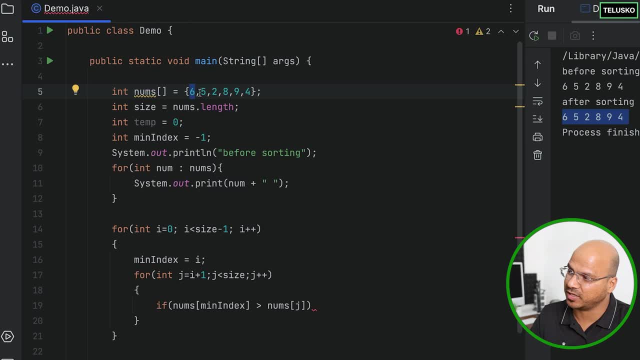 than five, then everything works. But what if six is greater than five? In that case we have to swap. Now, okay, we don't have to swap. We basically have to change the min index to j, Because the new index you will get is j, So the new index here is one. Okay, So that's the min index. So what we are doing by doing this is: after the entire iteration, you will get the minimum value from this array. Okay, So that means, after this iteration, you will. you will know that two is the minimum value. 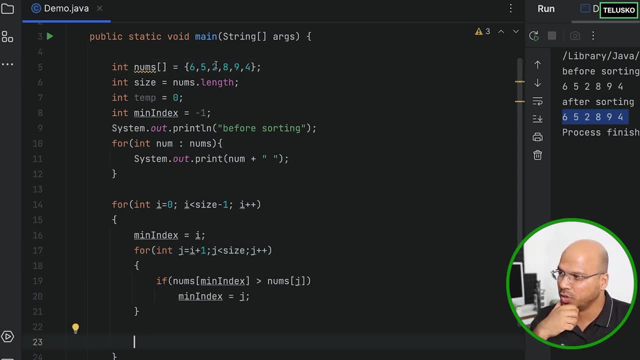 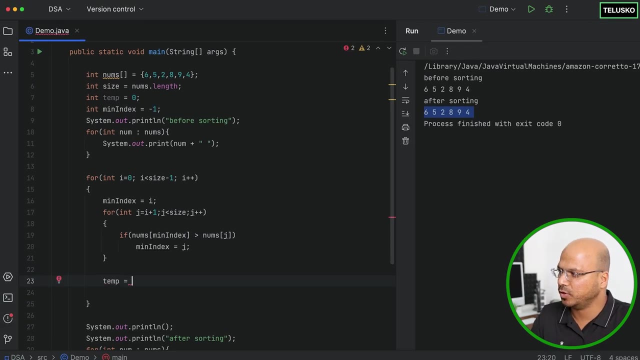 Now, once you know the minimum value, what you do is you swap two with six. Is that simple? How do you swap two and six? How do you know we have to swap six, because i is referring to six and the min index is referring to two. So we can simply swap them, So we can use a time variable here and we can put nums of min index and we can say nums of min index is equal to nums of i and nums of i is equal to i. 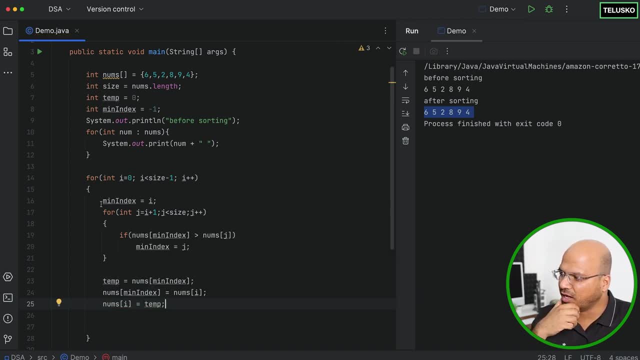 equal to 10. so basically, we just have to swap them. so what we are doing is, in the inner loop, we are just finding the minimum value and then, once you find it, you simply swap it with the min value which you're considering, which is the first value, and as the i value goes up, first you. 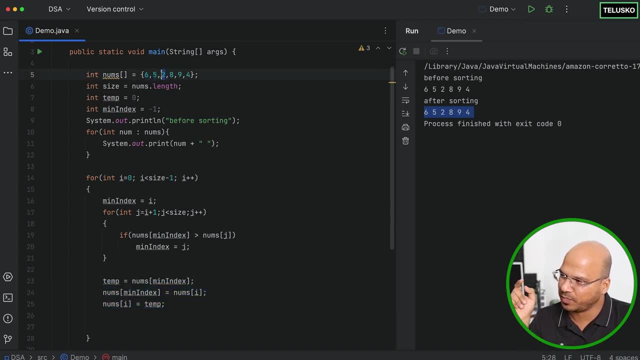 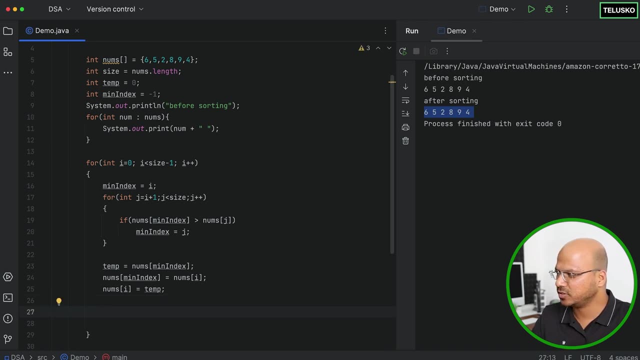 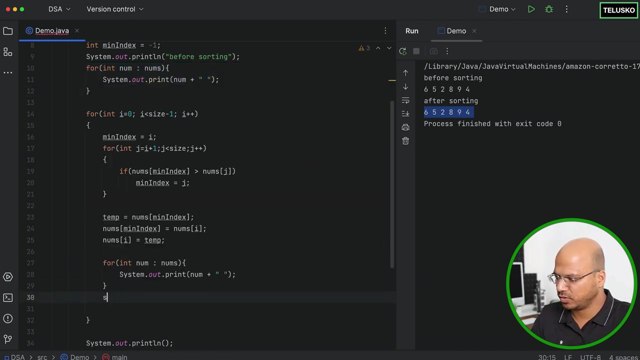 will compare with this, then you compare with the five and you compare, then you make two as a minimum after, of course, after the swapping. and what i will do is i will also print this- values after age iteration, so i can just copy this and paste it here and we also print a new line to get it.